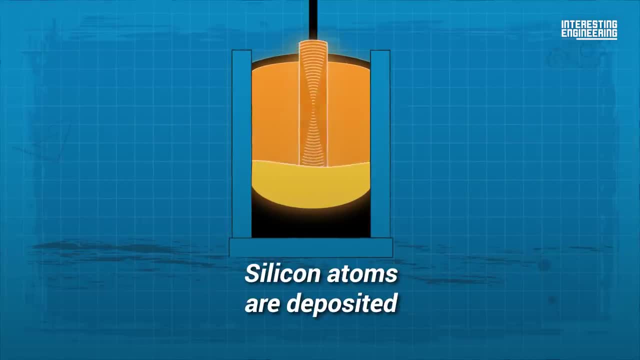 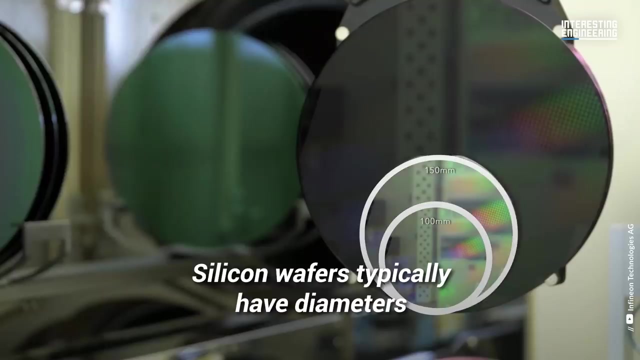 As the seed crystal is slowly pulled away, silicon atoms are deposited on the bottom surface. The result is a large cylindrical boule or a single crystal ingot of pure silicon. The boule is then thinly sliced into wafers. Silicon wafers typically have diameters of 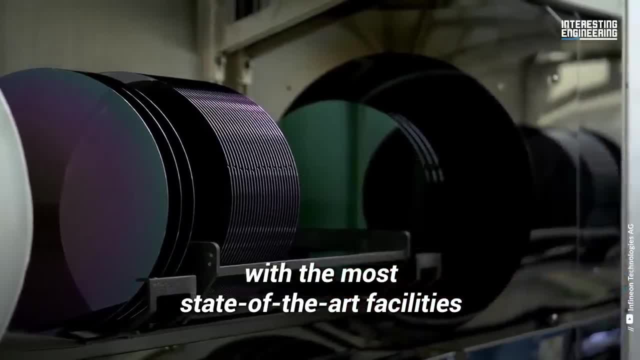 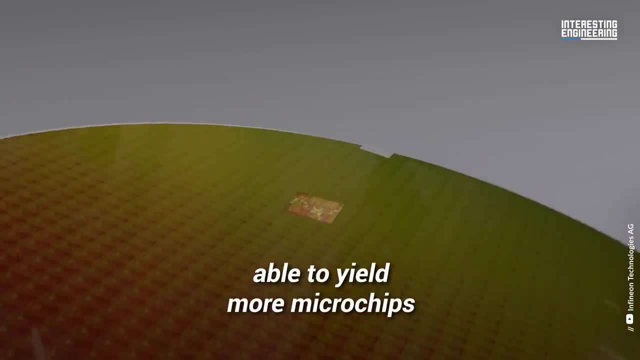 1 to 12 inches, with the most state-of-the-art facilities being able to produce wafers up to 18 inches in diameter. Bigger wafers are, of course, able to yield more microchips, such as silicon. The silicon wafers are also known as microchips. 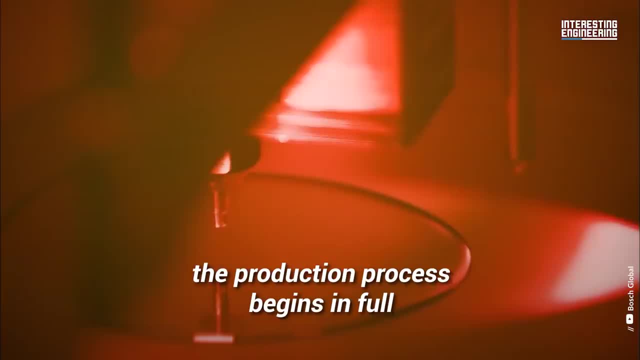 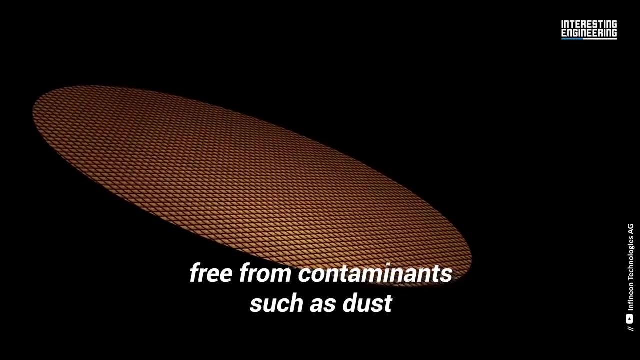 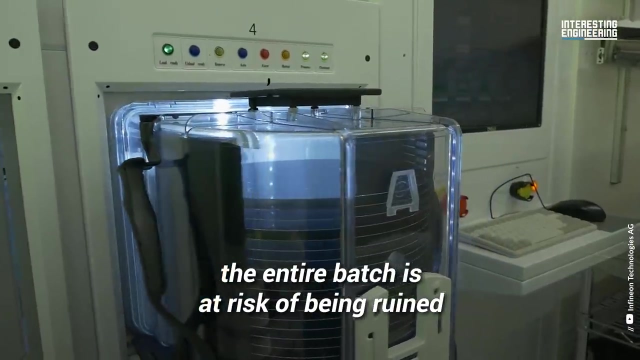 Once the silicon wafers are cut, the production process begins in full. Microchips are made in extremely sterile conditions, free from contaminants such as dust. If even just one particle of dust makes its way onto a silicon wafer, the entire batch is at risk of being. 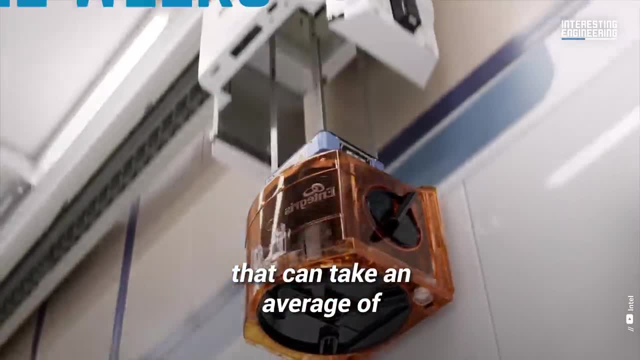 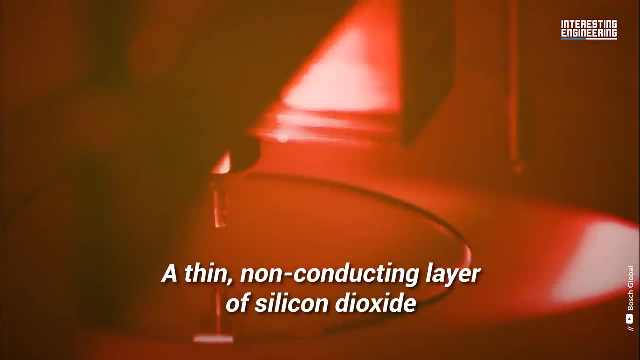 ruined. This would derail a process that can take an average of 12 weeks. The first step of the production process is deposition. A thin, non-conducting layer of silicon dioxide is grown or deposited on the surface of the wafer, Then the silicon wafer. 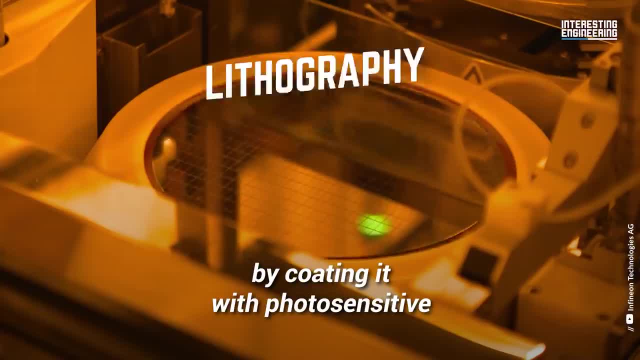 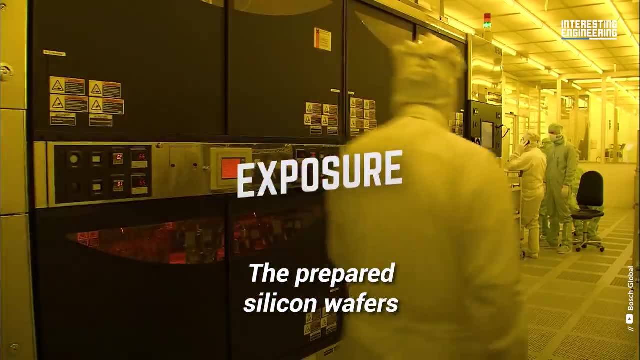 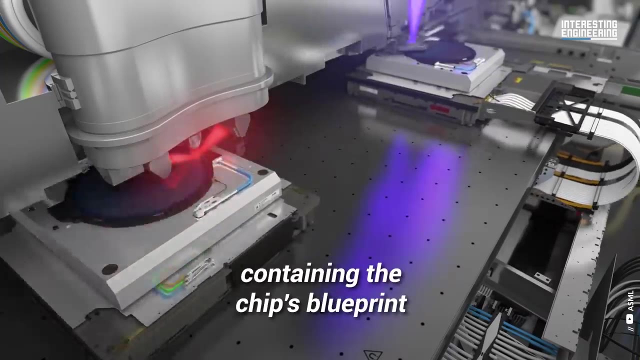 is prepared for lithography by coating it with photosensitive and light-resistant materials. The next step is very critical—exposure. The prepared silicon wafers enter a lithography machine and are exposed to UV light passed through a reticle containing the chip's. 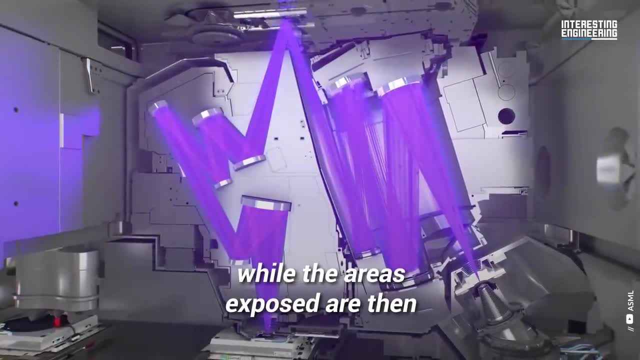 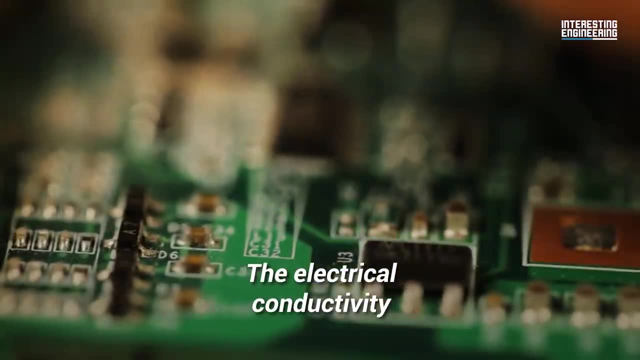 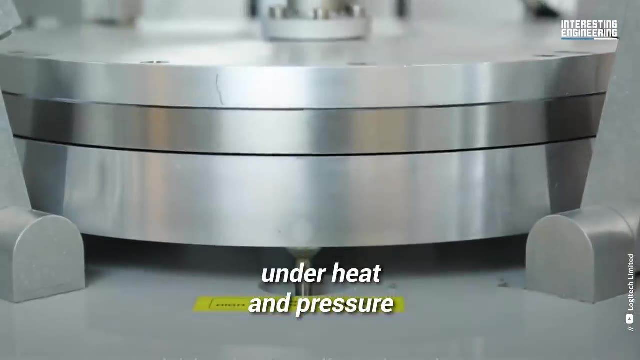 blueprint. The areas exposed to light are hardened, while unexposed areas are then etched away by hot gases to leave a three-dimensional microchip. The electrical conductivity of different parts of the chip can also be altered by doping them with chemicals under heat and pressure. This process can be repeated hundreds of times. 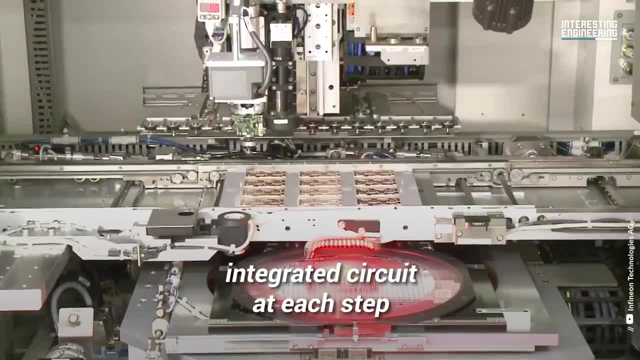 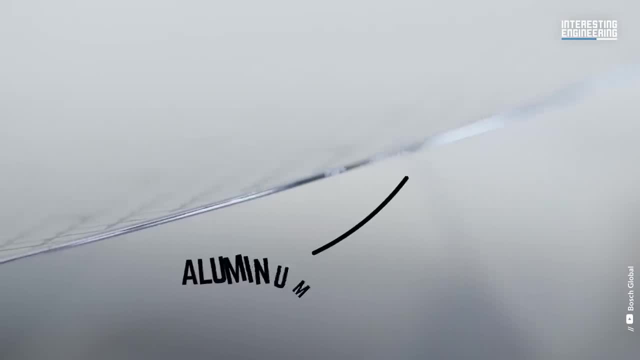 for the same chip, producing a more complex integrated circuit at each step. To create conducting paths between the components, a thin layer of metal such as aluminum is overlaid onto the chip and the etching process is repeated over and over again. The electrical